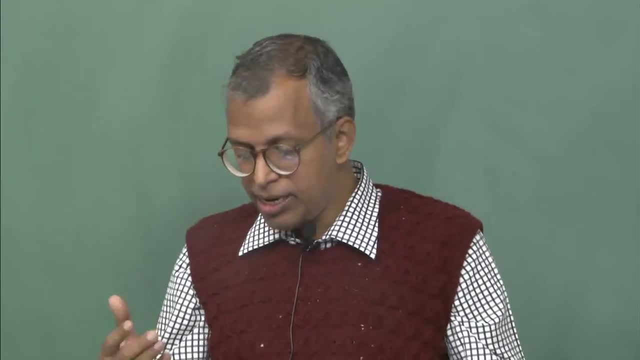 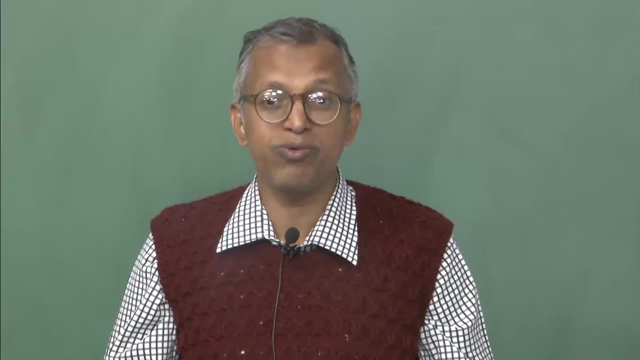 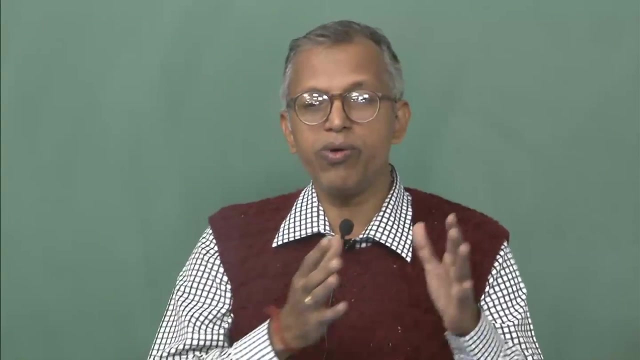 see how we can really carry out, which will be more realistic Still. we are doing some kind of- or we will be doing some kind of approximation as well, but that is good enough. that is rather better than the ideal one. So what we will be doing In this case, we will be looking at the losses incurred. 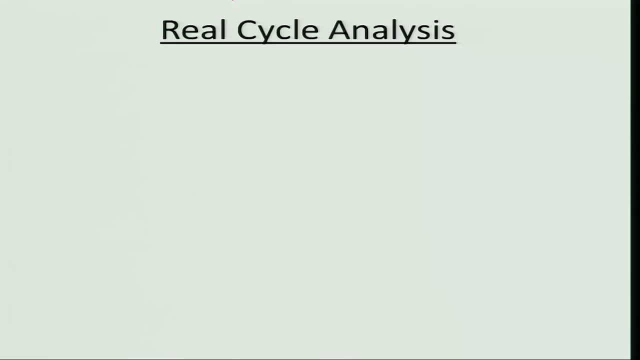 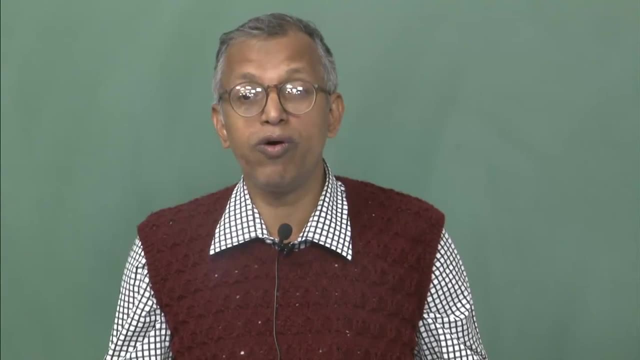 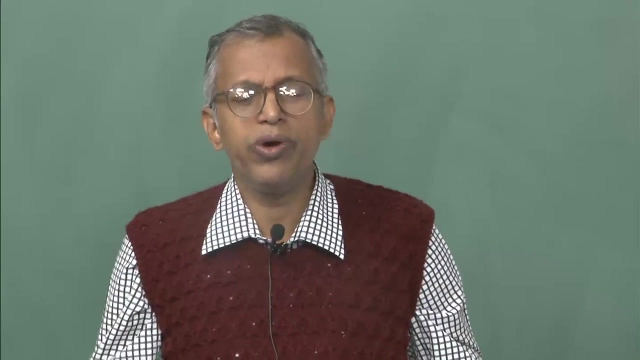 in the ideal, in the what you call real gas turbine energy, and we have not considered any losses in the ideal cycle analysis. However, we need to look at. So if you look at losses, all the losses kinds of, there are various kinds of losses. we can divide them into how: 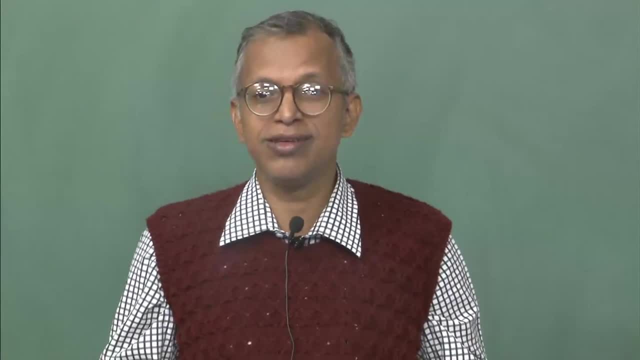 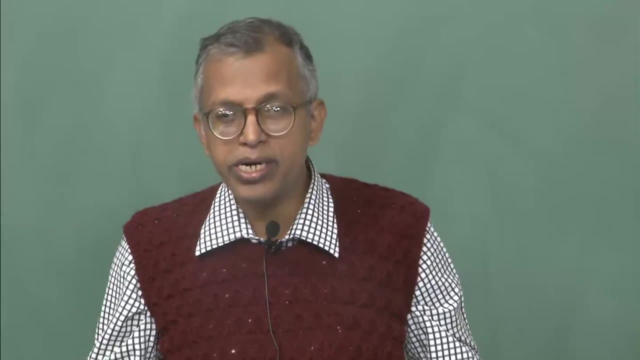 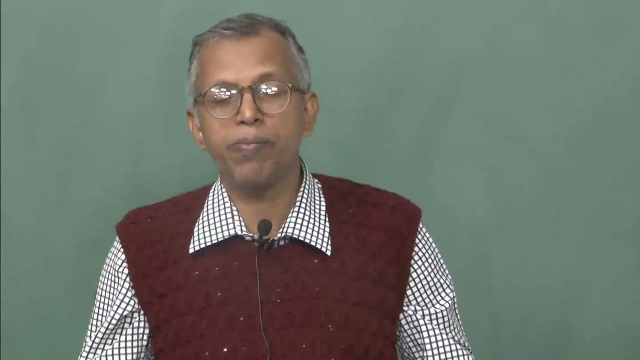 many categories. What are those losses? For example, flow is occurring in a air intake. It is occurring through the compressor or the turbo machinery, you know, turbine. That means there will be some losses due to frictional losses. There might be separation, there might be mixing. So those are losses. Beside this, 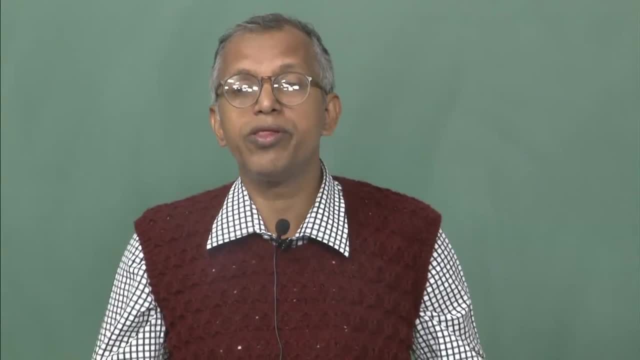 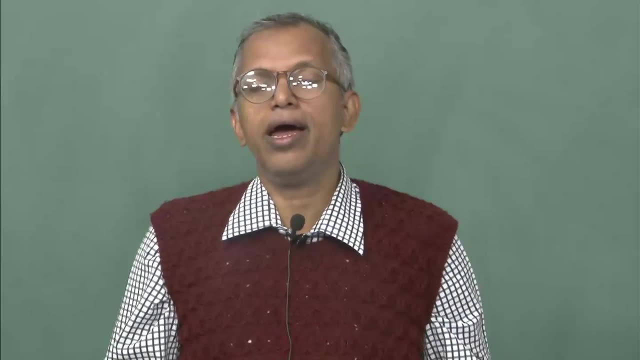 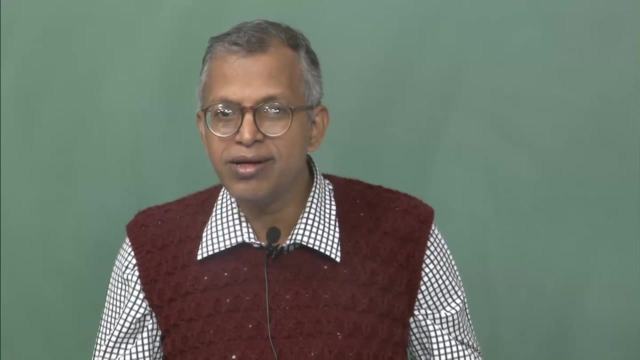 there will be some transmission, you know, and the transmission of power from turbine to compressor, turbine to propeller, and there will be all the power given by the turbine cannot be transferred to the compressor and there will be another kind of losses which will be basically due to the heat transfer. 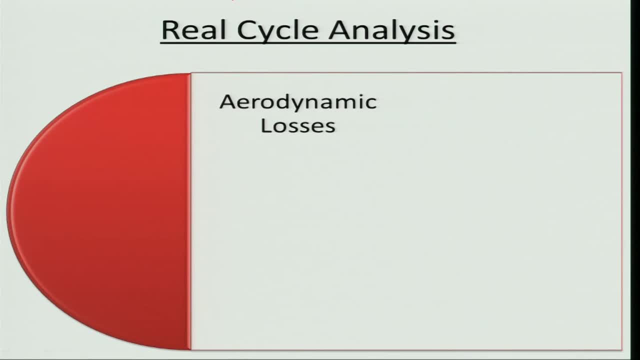 And we, because when the flow is taking place it is combustor, so it can be So broadly. it can be divided into three categories: One is aerodynamic losses, other is thermodynamic losses and the third one is the mechanical losses. right, 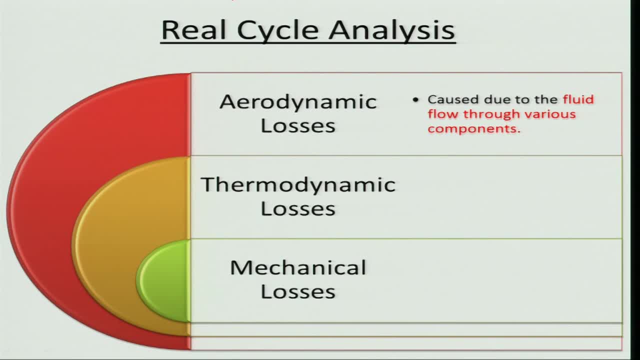 And aerodynamic losses. as I told, it is basically due to the fluid flow through various components of engine, which is quite complex in nature, particularly in turbo machines, And it will be adverse pressure gradient, like in compressor, air intake and other places. 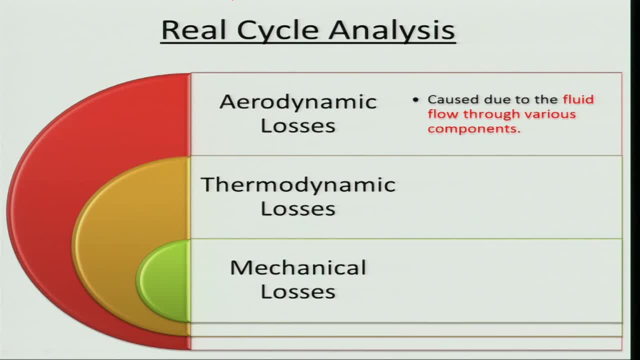 If you look at your combustion chamber, it is quite complex, particularly the main combustors, Even the afterburner. there will blob bodies, there will mixing, there will losses. So those are aerodynamic losses and thermodynamic losses is due to incomplete combustion of. 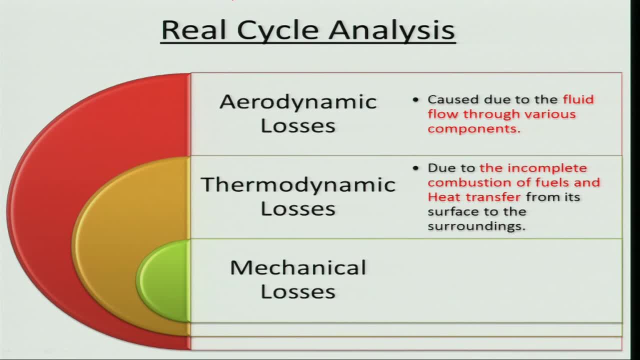 fuels right, Not that all the fuel you cannot really convert into the energy not possible in real situation. For example, if the fuel is because of the oil is taking place for because it will be operating over a wider range during its operation And beside this, 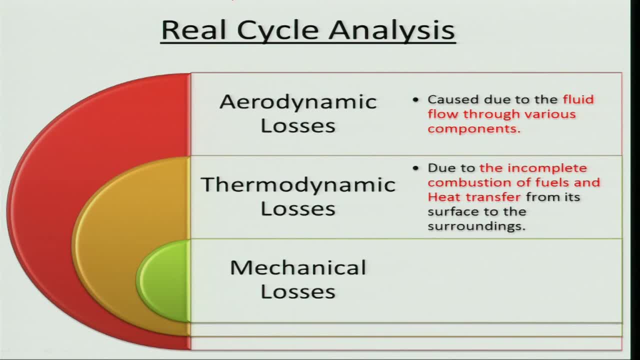 heat transfer is inevitable. although we have assumed there is no heat transfer, it is inevitable to the, you know, from the component to its surrounding And, as I told you, the power transmission you know has to be taken place from turbine to the compressor, to the propeller and then 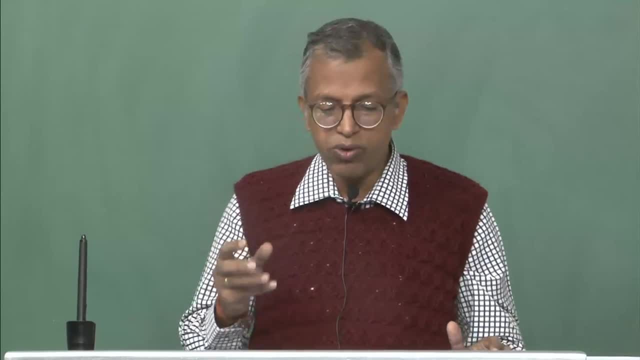 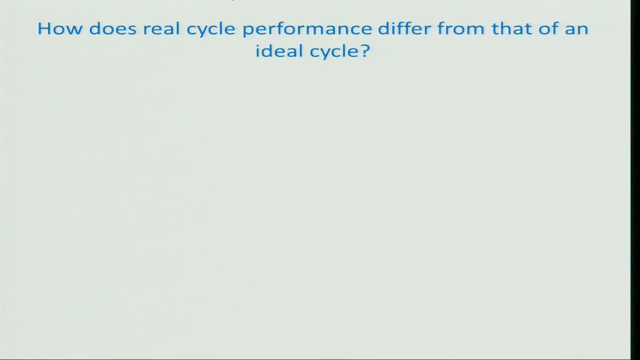 there will be some losses. So all these losses we need to now consider and let us see how we will be working with it. And let us ask question: how does the real cycle performance differ from that of an ideal cycle? What are the those things? If you look, 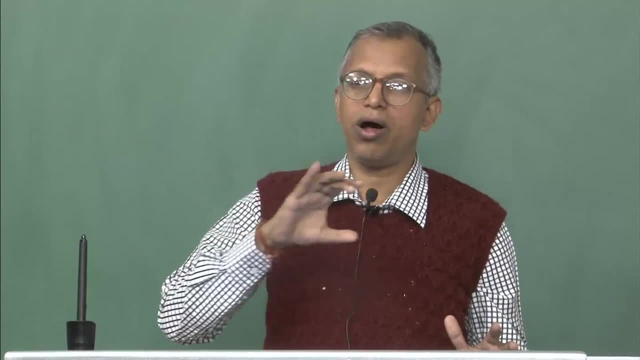 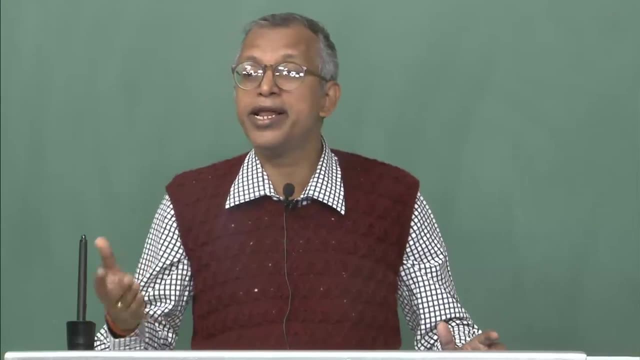 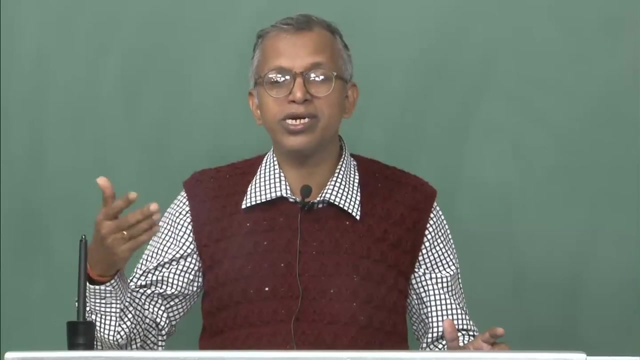 at. we have assumed in the your all the components you know, having the all same properties, like air. we say air standard, ideal cycle, right, But in real situation it is not the air alone. from the combustor onwards will be the several other combustion products, fuels and other things will be coming. number one, Number two: 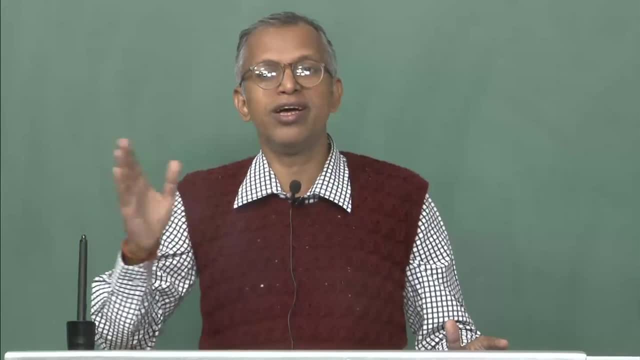 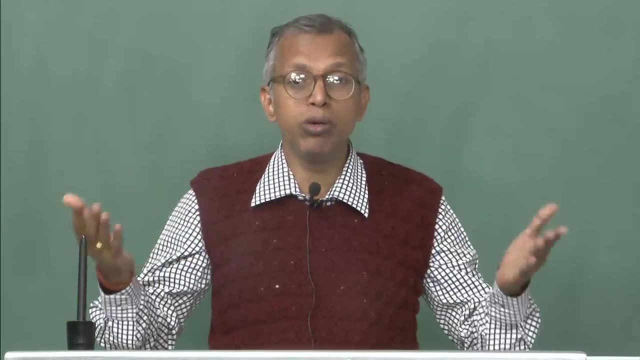 temperature is changing from intake to the nozzle exchange and, of course, peak temperature will be occurring in the combustion chamber right. So therefore, the C? p values will be changing, gamma will be changing, several kinds of things will be occurring which we have not considered right. 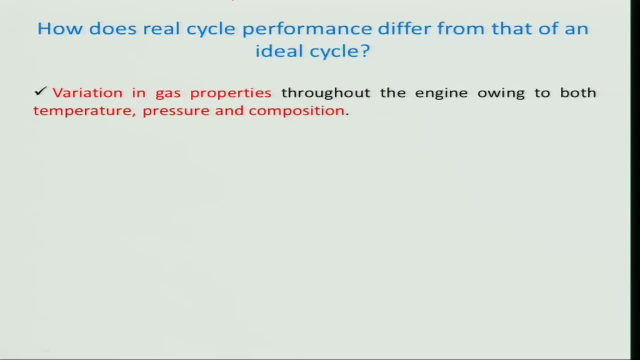 So this is the ideal cycle. So, as I told you, variation in gas properties throughout the engine, going to both temperature, pressure and compression: It is not the compression which is changing, but also the pressure and temperature is changing. So and non isentropic. 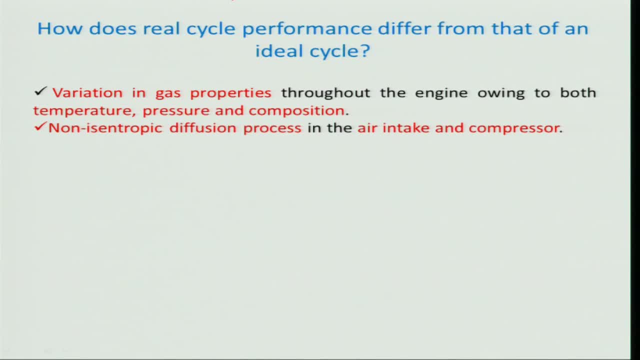 diffusion process in air intake and compressor. Similarly, non isentropic expansion in the turbine and nozzle right, But in real you know like air intake and compression. Similarly, non isentropic expansion in the turbine and nozzle right, But in real you know like air. 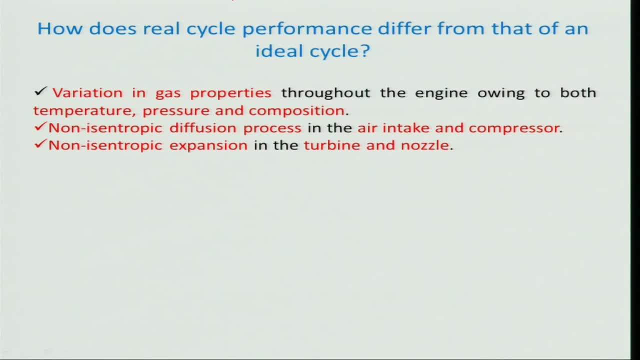 intake and compression. Similarly non isentropic expansion in the turbine and nozzle right. So these are the ideal situations. we have all consider isentropic processes right both for the compression and expansion. So change in kinetic energy and potential energy between 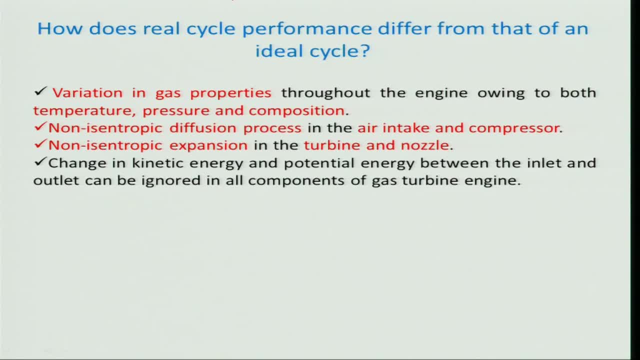 the inlet and outlet can be ignored. all of the components of gas turbine engine, Of course. that we will be considering because we are interested to look at the total one. And of course, potential energy is not very important, particularly for case of gas turbine engine. because all will be standby in similar level. But when you use the gas turbine in a turbine engine, completely, totally and completely different than after all, this internal combustion can be generated by the main blow. I have provided a liquid going deep endales large French turbine. 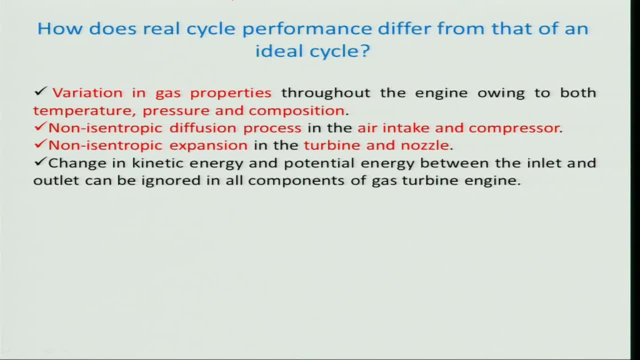 susceptibility of air intake and combustion, natural energy generation and motion resistance, suspension, the centrifugal compression and centrifugal turbine we need to worry about, but those contribution will be very, very less. But in case of steam turbine and other thing, 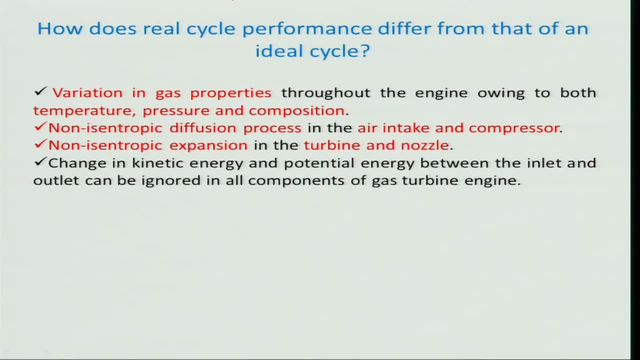 you might be knowing, potential energy plays small role, but here, in this case, we need not worry about it. So there is a another one which, of course, I would not be discussing, but you can note that bleed air extraction from the air intake. 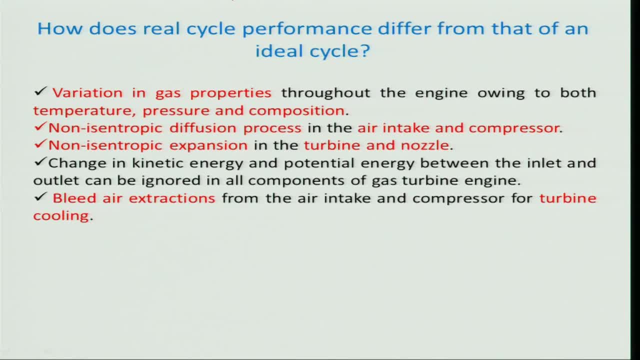 and compression, you know, for turbine cooling, because we need to cool the turbine right And it is basically the, this air, which will be causing problem in case of your air intake and compression right. You will just transfer this problem. problem due to what Problem? 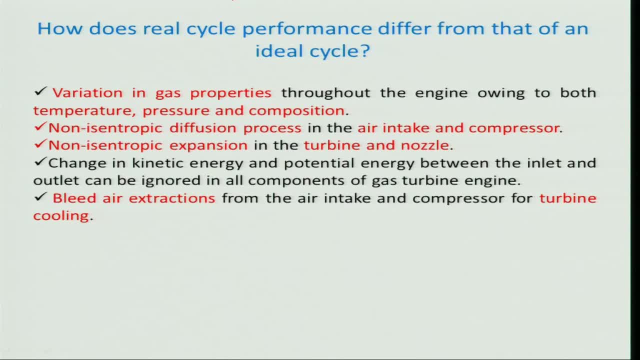 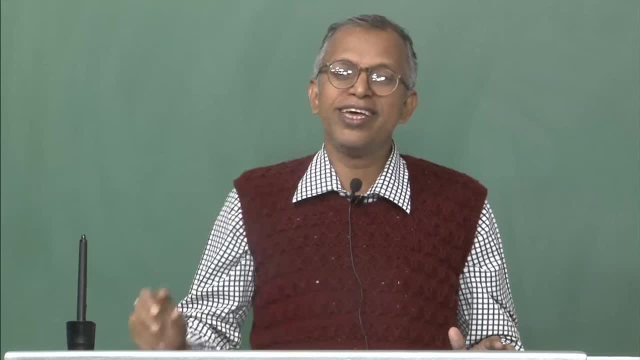 due to surging flow separations and other things, due to adverse pressure gradient in case of air intake and compression. So which are the problem? now you know you will be using For cooling the turbine. it is the win-win situation kind of thing. right, That is the. 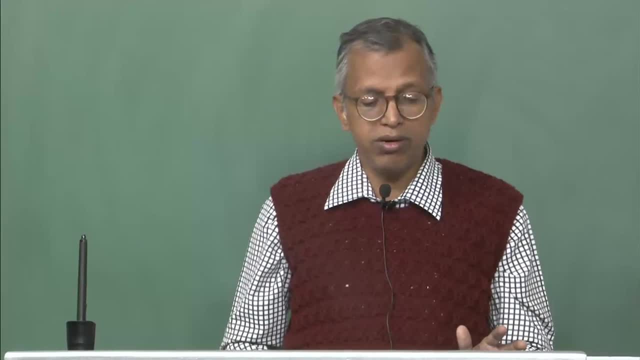 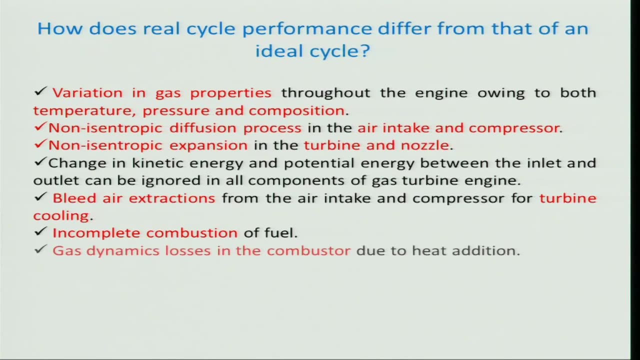 kind engineers they have developed. you know how to overcome the problem. at the same time solve another problem. So: incomplete combustion of well gas, dynamic losses in the combustor due to heat addition, the flow in the exhaust nozzle may not be fully expanded to the ambient. 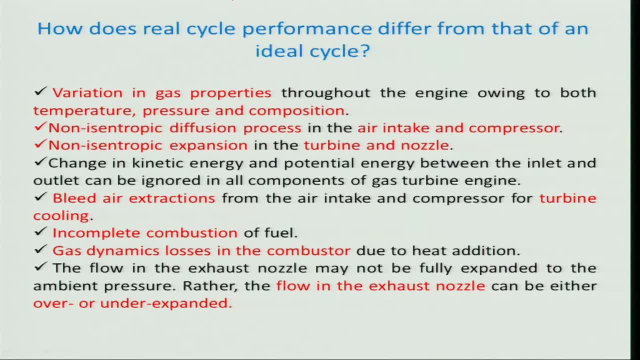 pressure. Rather it will be over expanded, under expanded, depending upon its- you know- older operating envelope. If you look at gas dynamic, we have already seen that Rayleigh flow. you know that is basically- we have already talked about it- how it will take care of whenever it is addition. 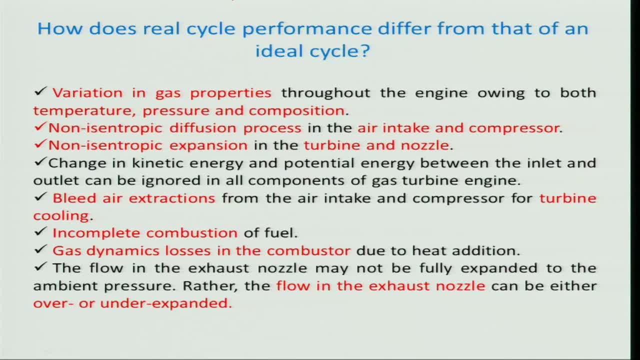 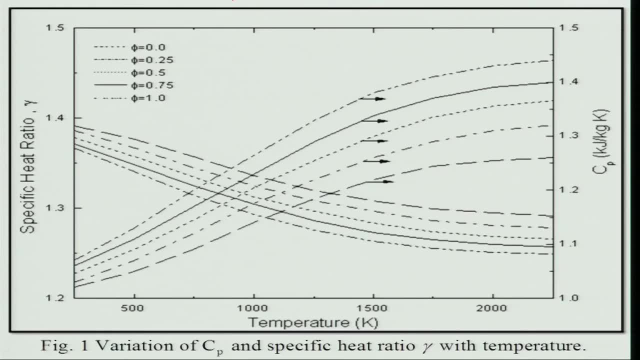 will be there. there would be losses in the pressure, total pressure. So let us look at how this C p will be varying with the temperature, because across the engine it changes from temperature: 300 kelvin to. it can go to even 2000 Kelvin, right, And 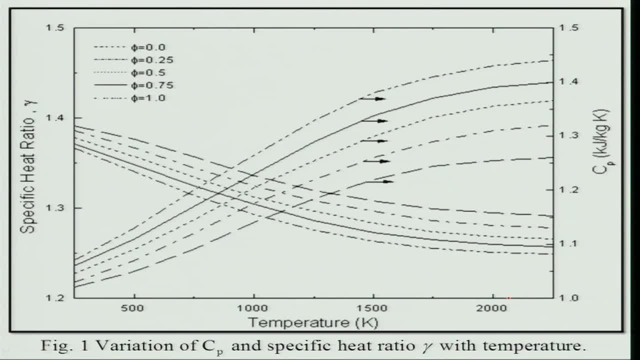 this water will be added to the Overall amount of total energy meals, which will be a ambient Kelvin, particularly after 1, is there. So if you look at the C p values, you know it can. it will be dependent on phi. What is this phi? Phi is basically equivalence ratio. 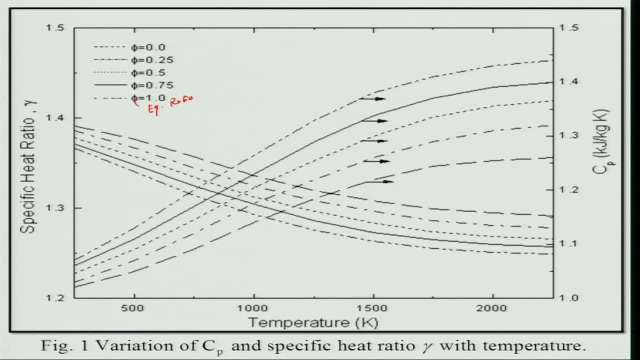 equivalence ratio, which we have already defined. So if it is 1, you will get a higher C p values. and keep in mind that the C p I have shown these are the C p values. C p is increasing with respect to temperature. That means it is increasing and, as you are having what you, 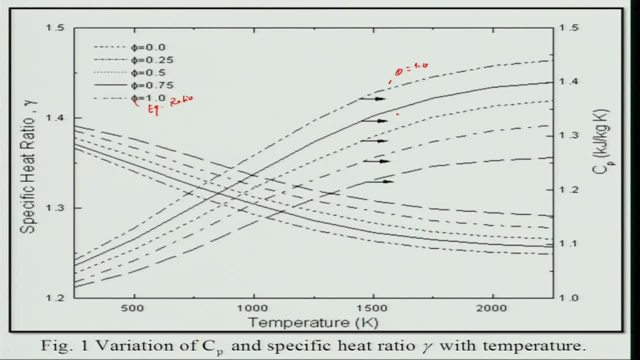 call 1, and this is phi is equal to 1 and as it decreases it become a 0, you know this, phi is equal to 0, the smaller one. But whereas the specific ratio gamma, that is C p by C v, right, it is decreasing with respect to the temperature for all equivalence ratio. 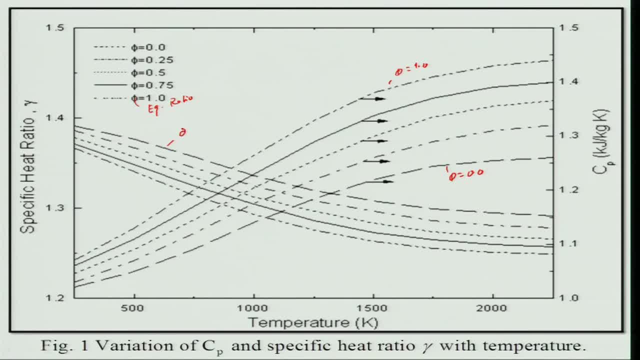 and keep in mind that this is basically phi is equal to 0 and this is phi is equal to 1 and it is just opposite of that of the C p right. So that means we need to take care of while analyzing the real cycle, because each components there will be change in temperature, But however, 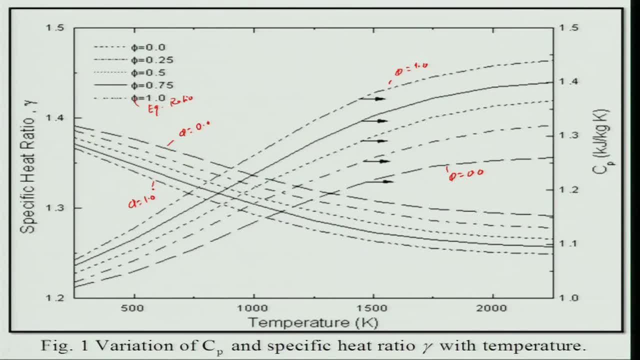 for computer program one can do this thing, but for hand calculation will be not easy because it will be very cumbersome. So you have to keep in mind that this is basically phi is equal to 0 and this is phi is equal to 1, and it is just opposite of that of the. 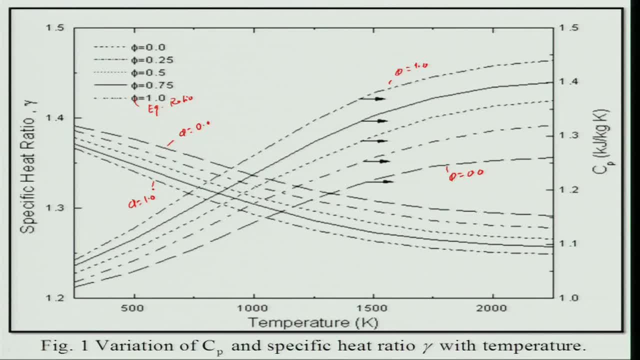 C, p, Why? For air intake there is a change in temperature. Now I will have to calculate along the air intake how it is right. Similarly in the compressor or combustion chamber. it will be very, very difficult job do a hand calculation, But in computer program I can have, because 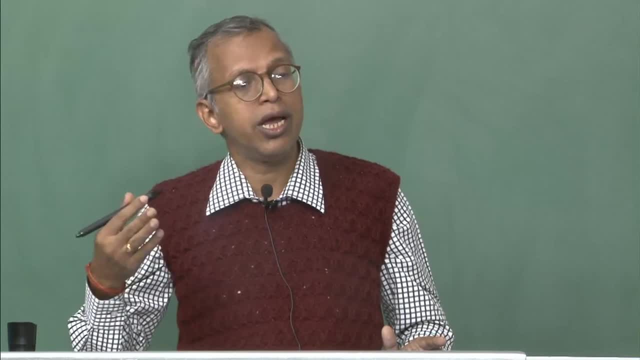 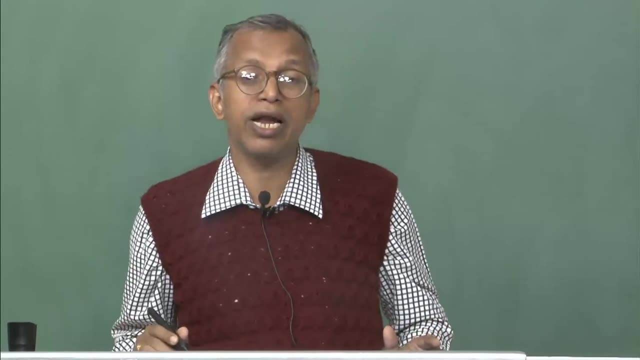 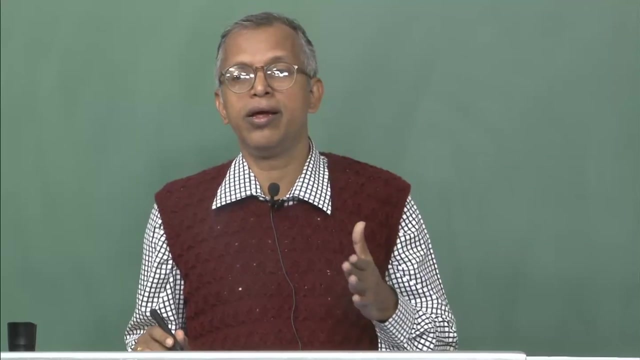 C p is a function of temperature- we can get coefficients- and it is also a function of spaces, right? It is dependent spaces for methane, for oxygen, for some other, then you will have to calculate average C p. So it is a quite cumbersome. Therefore we will be using till compressor 1, gamma right. 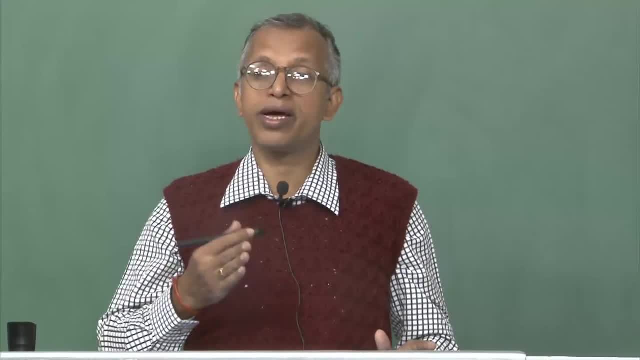 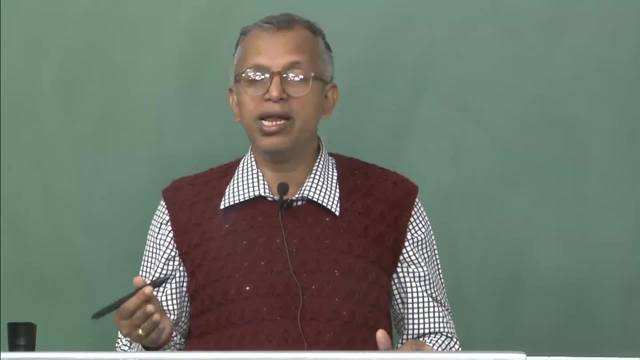 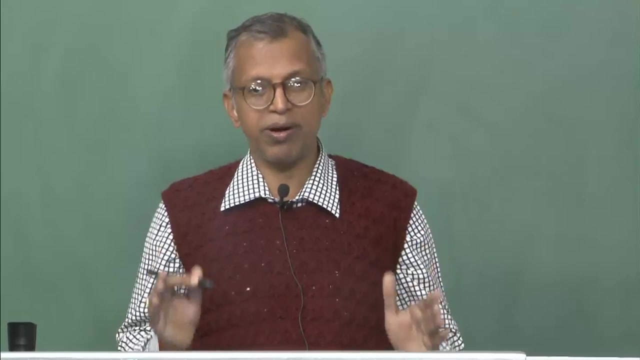 that is gamma 1.4, and for the combustor onwards we will be using another gamma right, gamma g right And similarly C p will be using 1.005 kilo joule per kg till compressor, exit of compressor and inlet of combustor. onwards we will be using another gamma g. So this 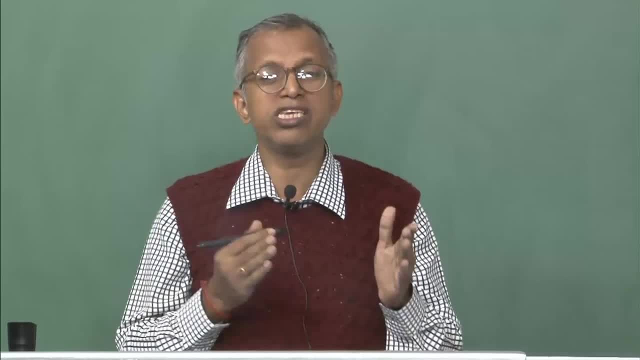 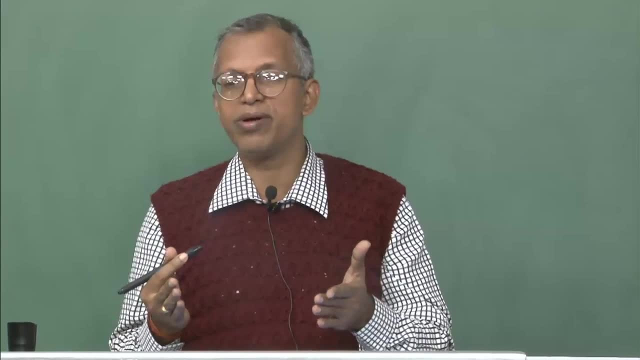 will be using another C p. That means 2 C p will be using C p a, C p g. That is for the simplicity. Again, we are doing an approximation here, just to make it problem tractable which can be solved by hand, right. 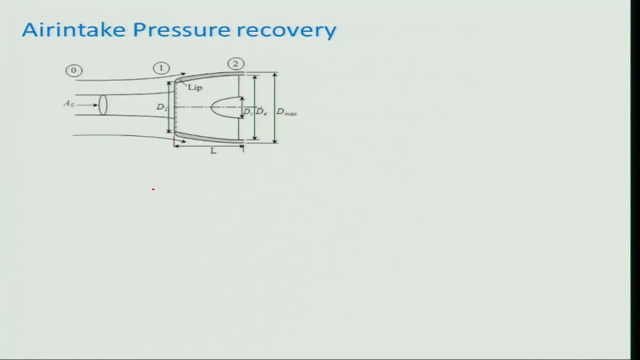 So let us look at air intake pressure recovery and if you look at, this is an air intake and these are the lifts right in which the air will be entering into the air intake. If you look at, there is a divergence of the stream line. What it indicates? What it indicates. 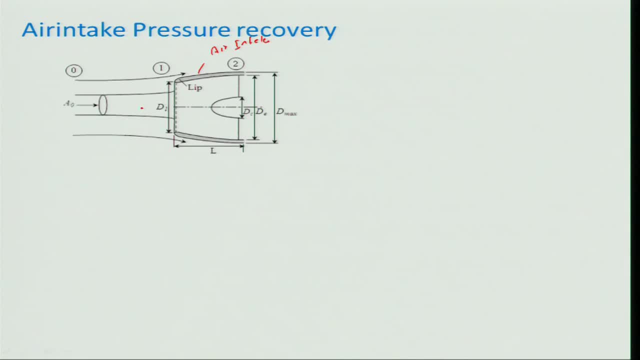 There is a divergence here. you know it is diverging. What is the indicate? Do a continuity, move balance. you know mass balance. If you do, what will happen? Area is in the air. what will happen? Area is increasing If area increasing. what will happen If keeping. 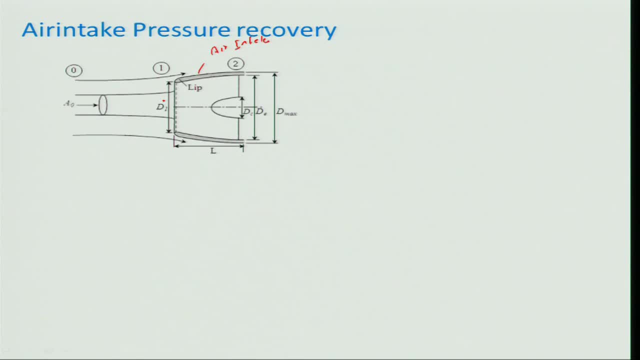 the density is remaining same, so velocity will be decreasing. That means this is deceleration, right, or diffusion you can call, And this is what you call external diffusion, external compression you can say, because there will be increase in static pressure, right And 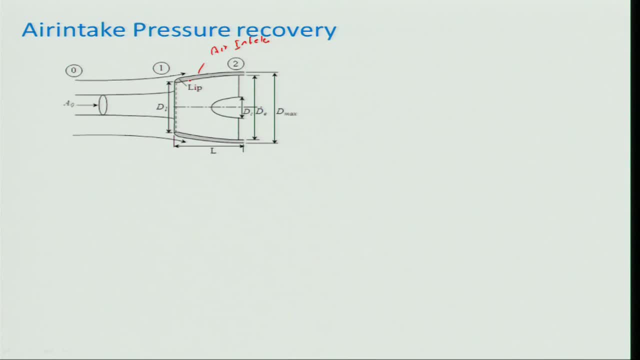 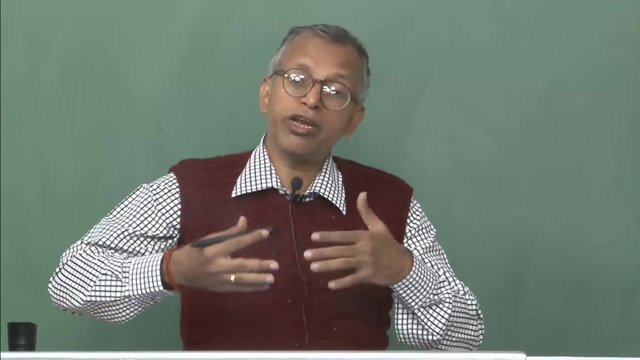 of course. however, it is going through the when it is entering. this is known as internal compression, Because if you look at air intake is a compressed. you know air getting compressed because decelerated right, the flow is being decelerated And there might be a situation where it will be. 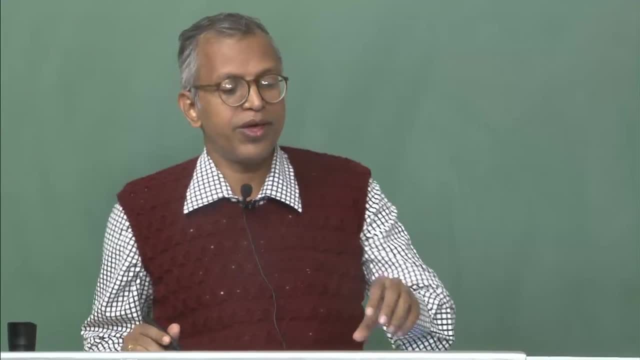 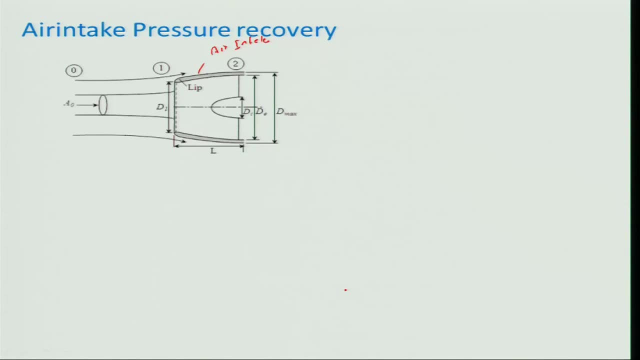 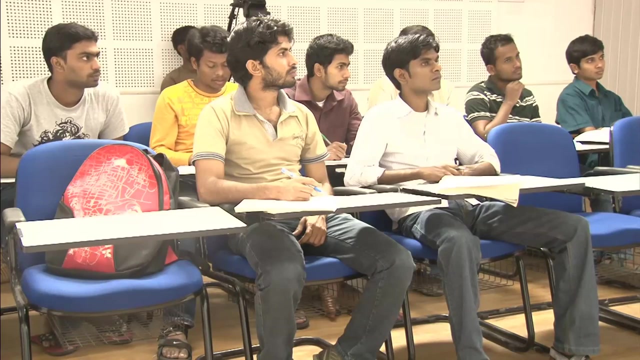 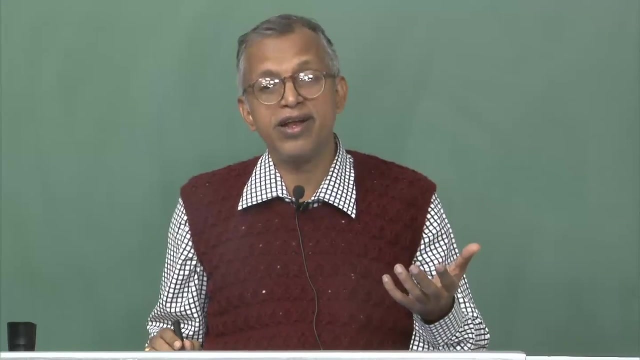 other way around. It will be accelerated in the, your external portion, 0 to 1, right, Will it really occur When, For example, under what condition? Standing all the way around, or it is about to take off, Or it is climbing, you know, at that kind This will be, you say. 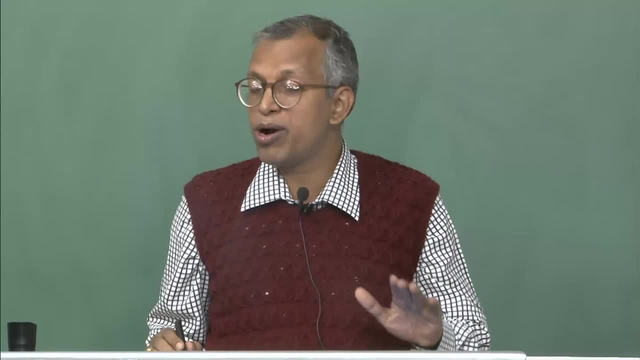 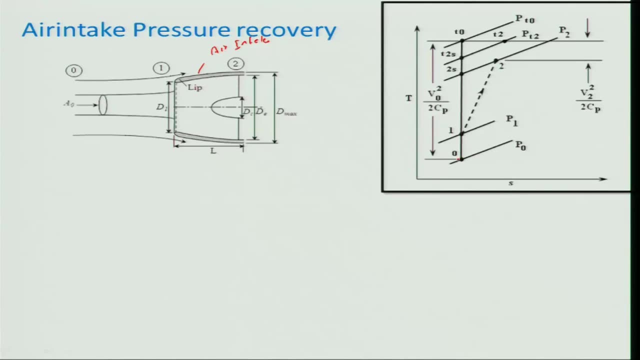 different This streamline if you draw it will be wrong. so I am not going to discuss, but you please think about that right. So now, if I look at processes in T-S, what is happening? this P naught is your the pressure. static pressure, freestim static pressure. 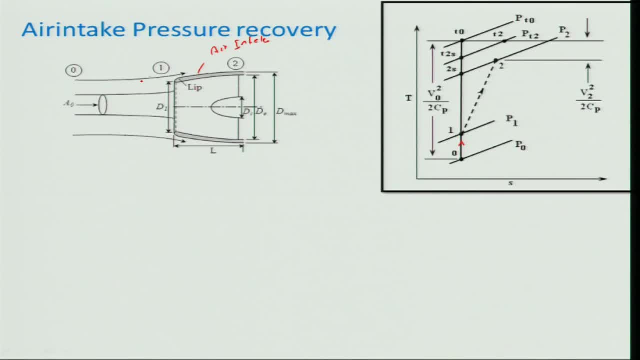 And there is a compression, and this is compression 0 to 1, right will be what? Isentropic compression, right compression? Am I right? Can I say isentropic? Can I say or not? Because there is no surface? 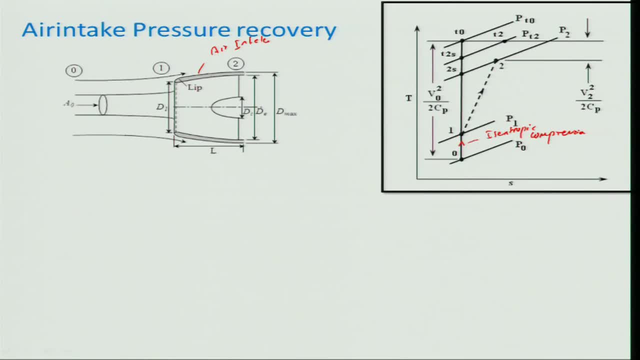 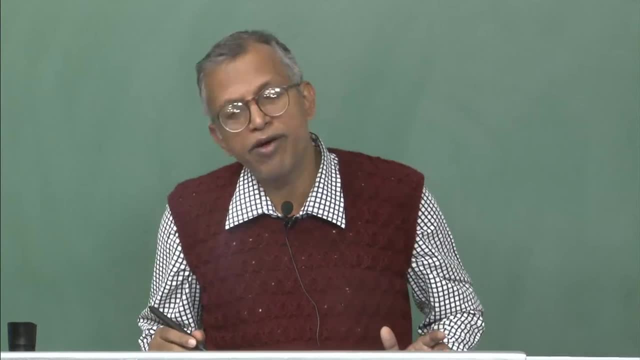 and also this compression is, the heat losses will be very, very low, So adiabatic and irreversible, because there is no losses in friction and solid surface is not there. So therefore it will be like this isentropic compression, But whereas these process, if you look at 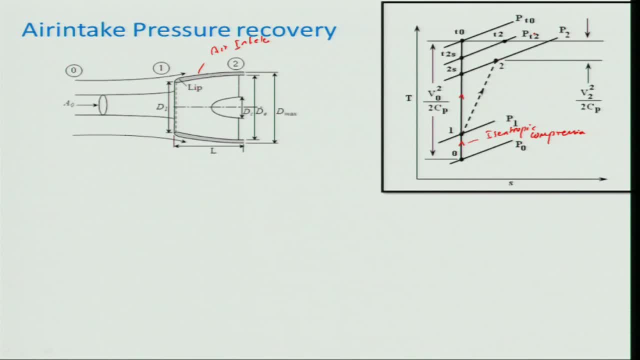 p 1 to p t naught or right. if you look at p t naught or t t naught, this point is equal to the t t 2.. So this process is basically the isentropic compression right, But, however, as the solid surface is there, so it will be having a lower pressure over here. p t naught. 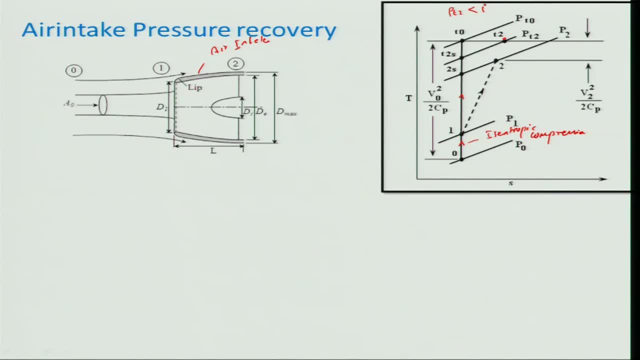 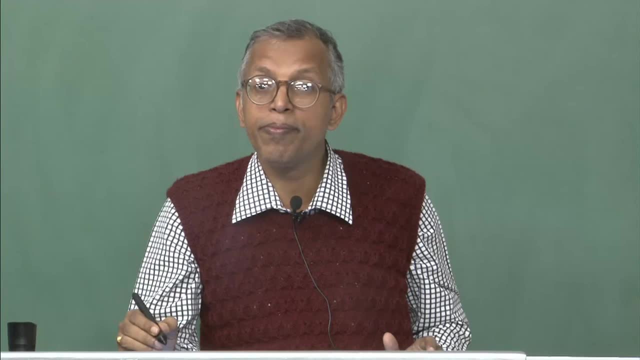 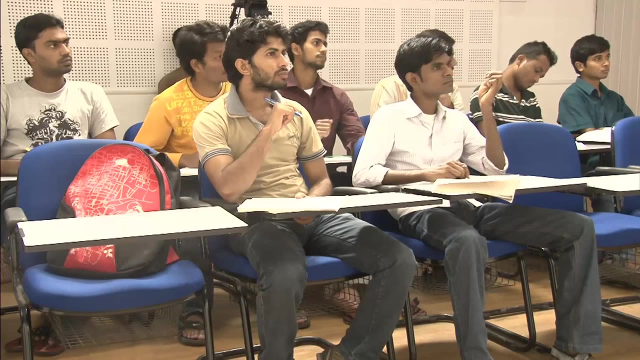 or t t 2.. That means p t 2 is less than p t. naught right, agreeable, disagreeable. It is not isentropic. This is not an isentropic process, Whereas the t 2 s. I am saying this: 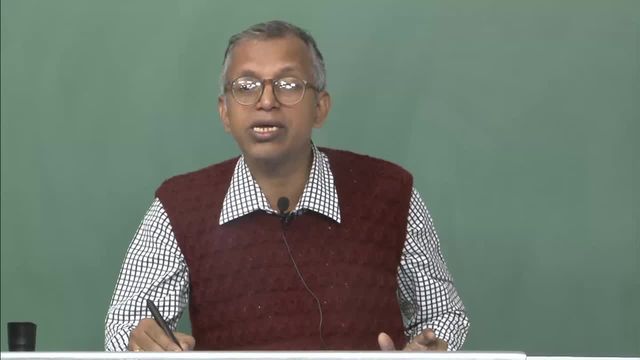 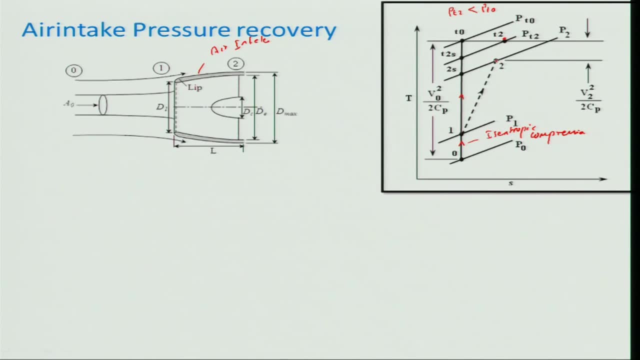 is isentropic s for isentropic I am using, Whereas this is not isentropic. That means this dash line, you know, is not an isentropic. So and the pressure p 2 is the static pressure. 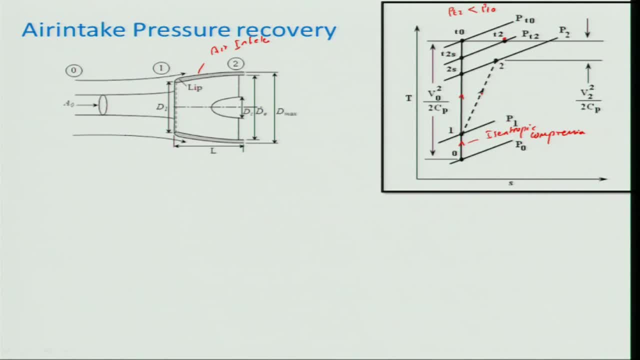 That means there will be, You know, change, compression, and I am indicated, I have indicated in the dashed line. keep in mind this velocity: v 2 square by 2 c p: this portion. v square by 2 c p: this portion right. 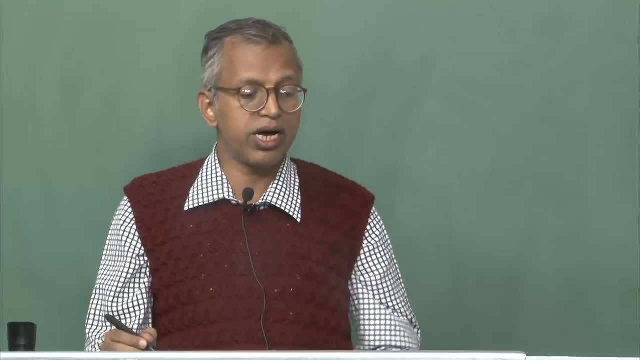 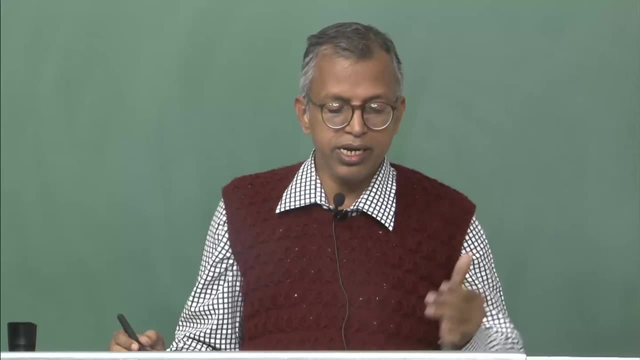 So what we will have to do now, how to handle that. that is the because, as I told, it is basically air intake to decelerate the freeze stream fluid smoothly to a lower velocity, either in subsonic or supersonic, And this is basically a subsonic diffusion. This is 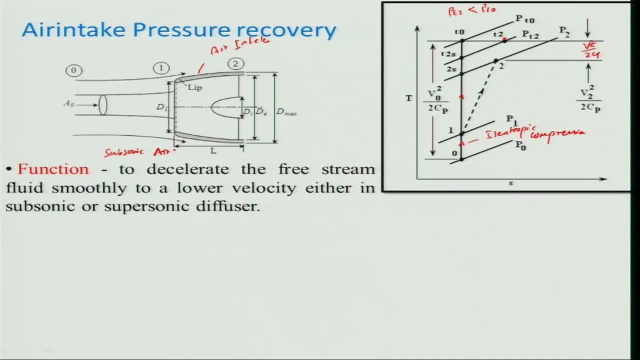 air intake, But the supersonic is there, then shock will be there. you need to take care of that, which I am not discussing, but it can be handled in the similar manner. I will be talking little later on. So what are the? 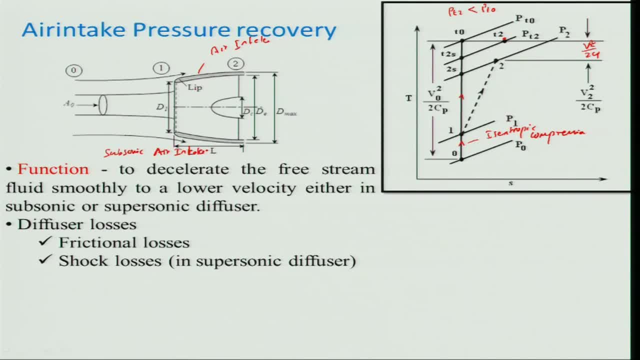 causes of losses: Frictional losses and shock losses in supersonic diffuser diffuser and air intake. both are interchangeable- can be used. So pressure recovery factor is basically: we need to define a pressure recovery factor that is basically ratio of average stagnation pressure at the intake. exit to the free stream. 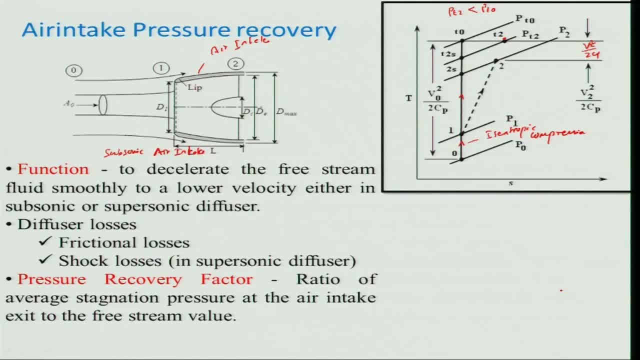 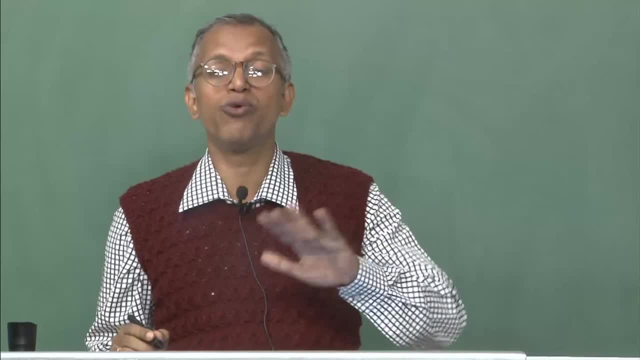 value. Why average? Because in each point you know it may be changing. So therefore I need to take average in real situation right Here. we are considering it to be flow, to be one dimension In real situation. flow can. 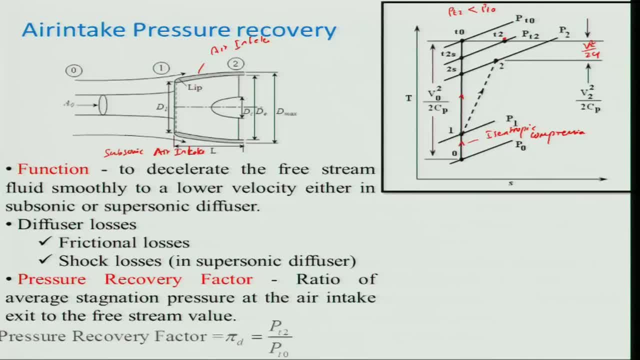 never be one dimension, So I will have to take average value. So therefore it will be P t 2 divided by P t. naught is nothing but pressure recovery factor. pi d: Always it will be less than 1, right. 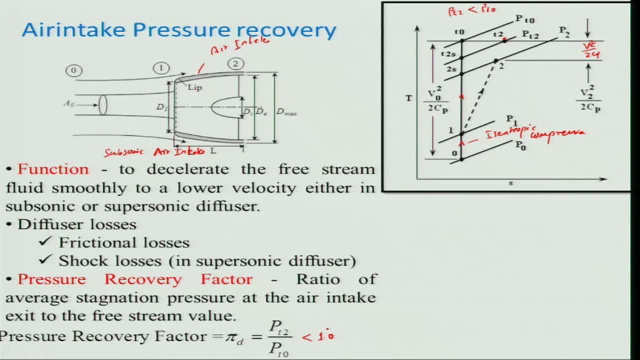 This will be less than 1.. P t 2 divided by P t naught. P t naught is here. If I convert all the total and that velocity V naught, you know P 1, P naught plus V naught square. 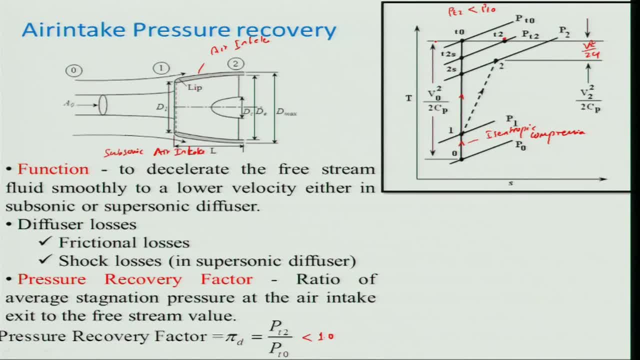 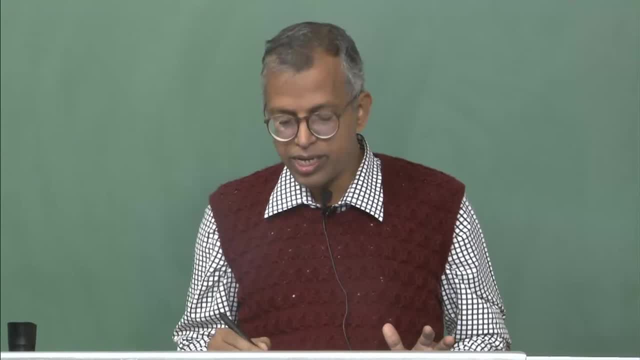 This is this portion right. Total will be P t naught. So P t naught is much higher, or rather not much higher. It is higher than the P t 2. So therefore it is less than 1.. 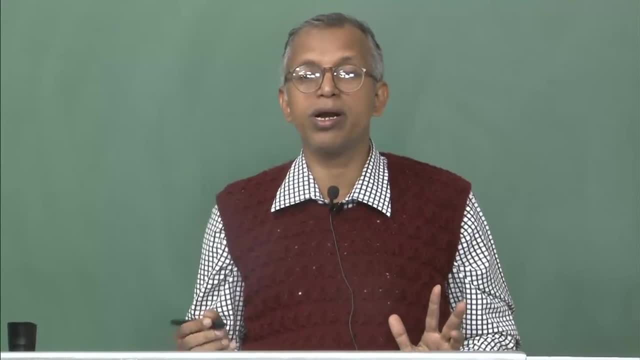 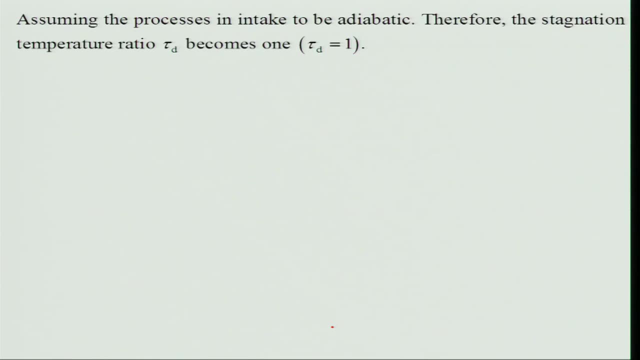 In ideal cycle, we have assumed it to be 1.. Pi d is equal to 1, but it is not 1.. Is that clear in real situation? So, assuming the processes in the air intake to be adiabatic, 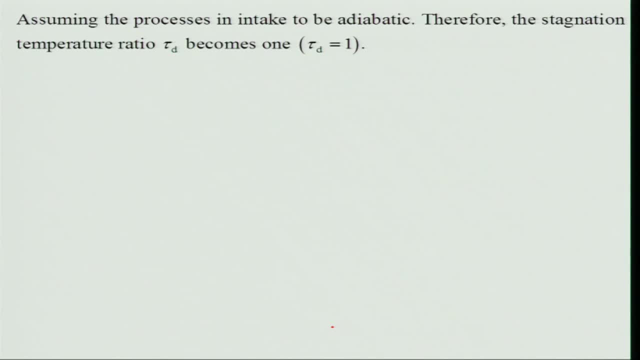 but, however, we are considering the process to be adiabatic in the air intake. Why? Because the change in temperature between the ambient and the adiabatic. So we are assuming the process to be adiabatic in the air intake. Why? Because the change in temperature between 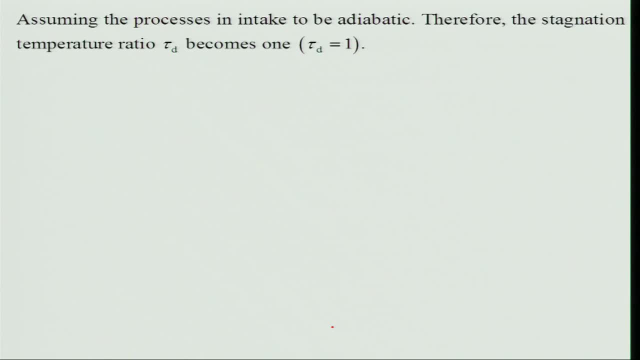 the ambient and the ambient, and this thing will be very, very low. So therefore, we are again in ascension, because it can never be in principle. So the P t, as I told you, P t 2 by P t naught actually will be less than P t 2 by P t naught. 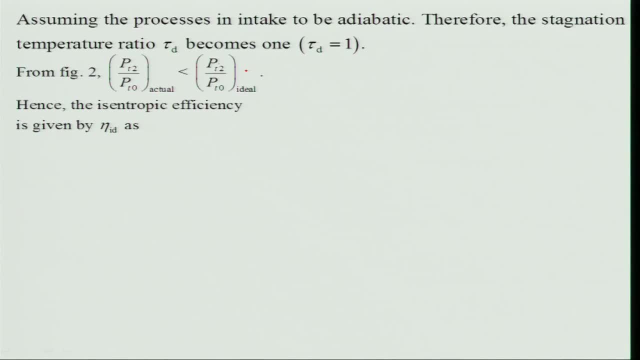 And P t 2 by P t naught is basically 1. in case of ideal right It will be less than 1.. Hence the isentropic efficiency is given by. we can define eta: i: d is equal to s 2. 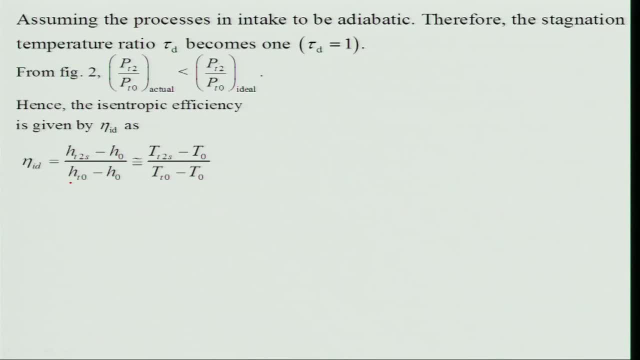 t 2 s. So this is minus H naught. that is the free stream divided by S t naught minus H naught, And we can assume again C p is same during this process, right? Therefore it is approximate. 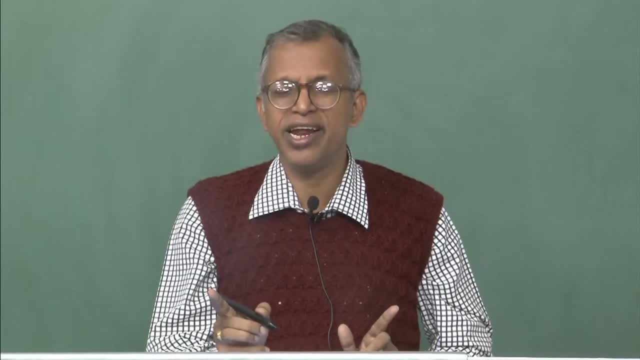 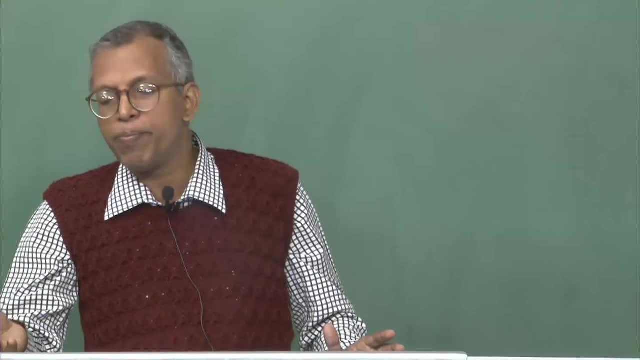 but it is not the really true, because C p will be changing right, As in our real analysis. we have assumed that C p will be remaining constant till the till the compressor exit. then we can manage this, Is that clear. 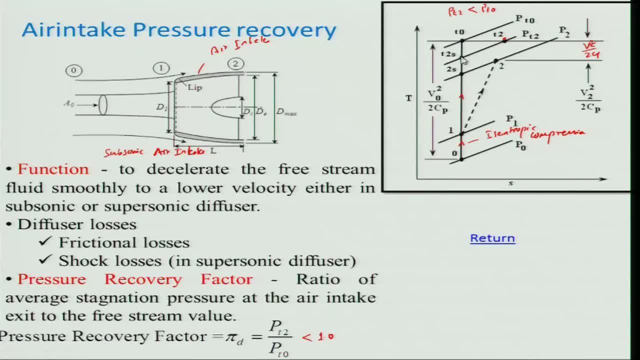 So if you look at, this is basically what I am saying. this is T t 2 s minus T naught and T t 2, T t 2, T 2, T t 2 s minus T naught, divided by T t naught minus T naught, right. 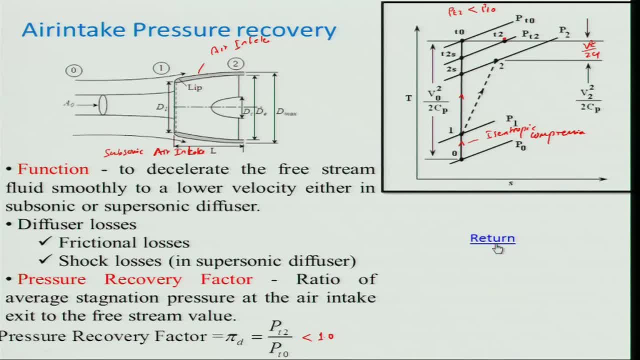 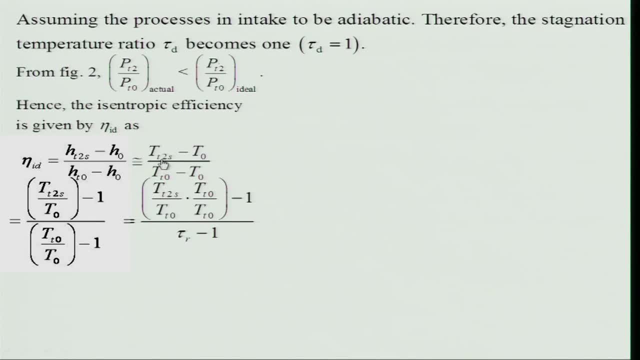 That is the isentropic efficiency for a air intake for an air intake. So if I look at this is basically T t. I can write down, I can divide this by T naught and I will get T t 2 s divided by T t naught, minus. you know, there is a little. 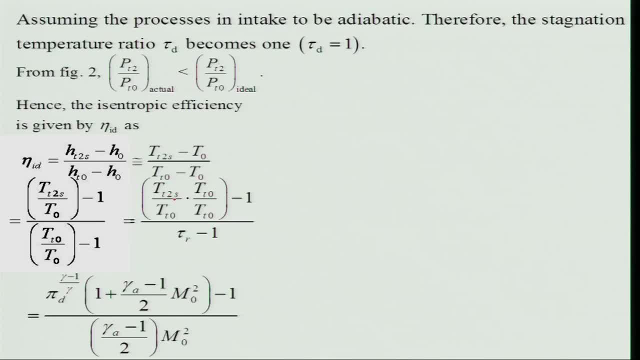 problem here. right, This is naught, So this I can write down. this is basically naught: T t 2 s divided by T, t naught into T t naught by T, naught right, And we know that T? t naught. 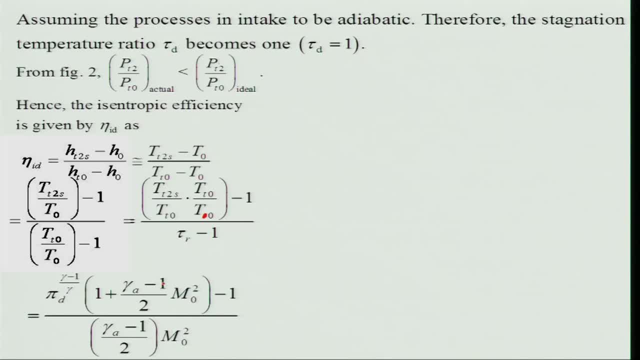 by divided by T, naught is nothing but 1 plus gamma, a minus 1. divided by 2, m naught square, is not it right? So this is the isentropic flow, because this portion is isentropic, right. So therefore, 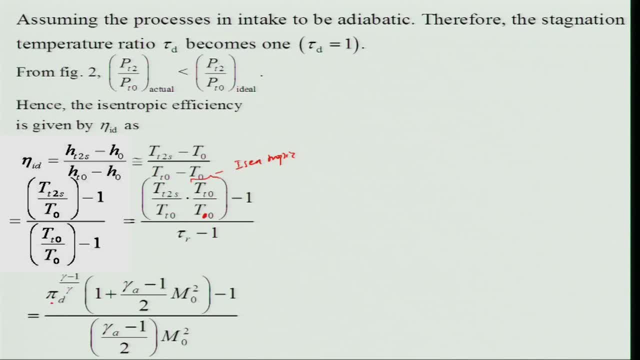 I can write down: and this is nothing but T: t 2 s divided by T. naught, this is nothing but pi d, gamma minus 1 divided by gamma. Keep in mind that here it is gamma a, this is gamma a. So and in, of course, if I put, this is basically: this is nothing but your tau. 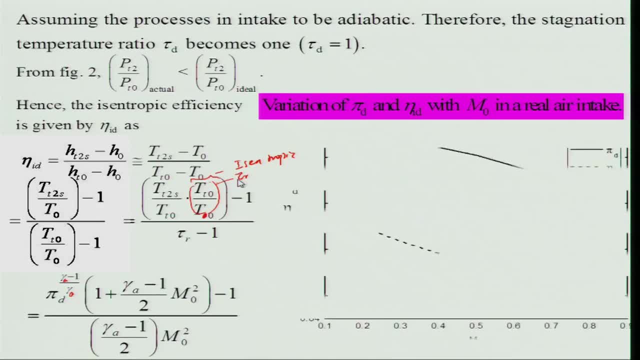 r this portion. So if I I what I am doing, it is basically eta. d is a, you know, function of flight Mach number and also it can be related to the pi d, If I know this pi d at values, because 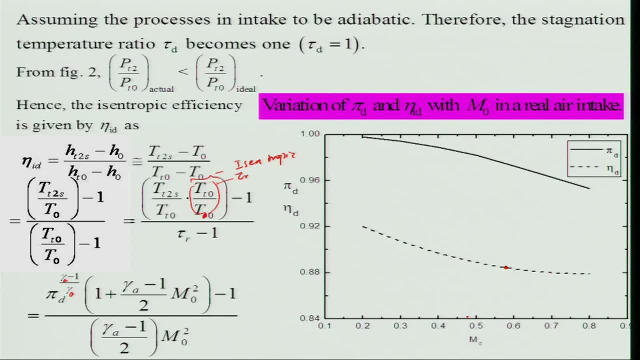 pi d when Mach number is very, very low, it is towards going to the 1,, yes or no pi d? Pi d will be 1, because there is no flow. I mean, like you know, it will be 1 kind. 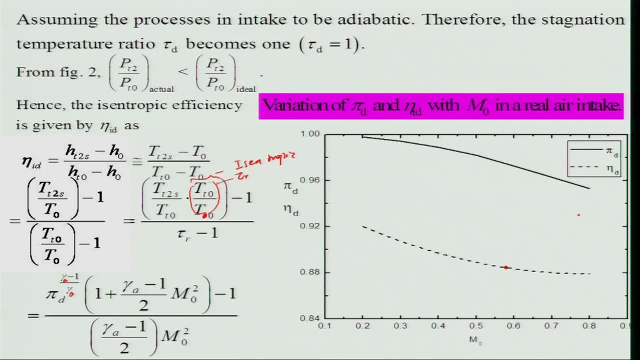 of it is going towards 1. but while decreasing with the Mach number. And if I know these values, I can get what will be the eta d, which is lower than this. So you can get a relationship between the isentropic efficiency for and air intake with. 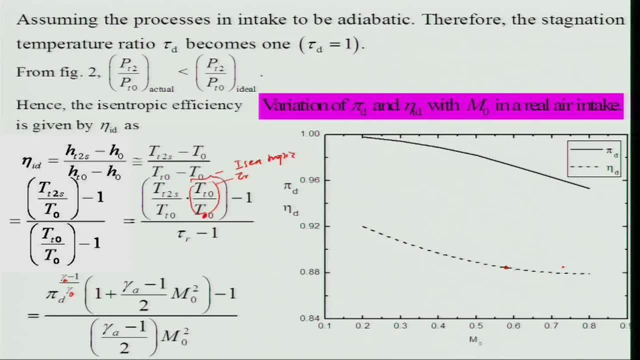 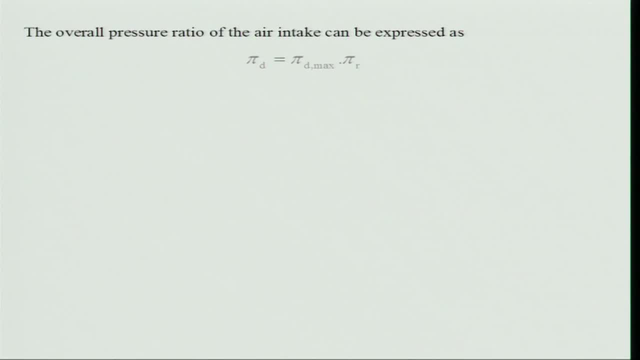 respect to the, what you call the pressure ratio, because the air or the diffuse, So the overall pressure ratio and the intake can be expressed as pi d, because we need to know this will be pi d maximum into pi r, and this is pressure is due to ram ramming effect. you 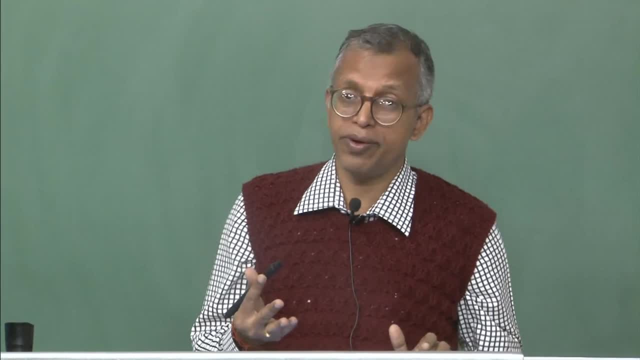 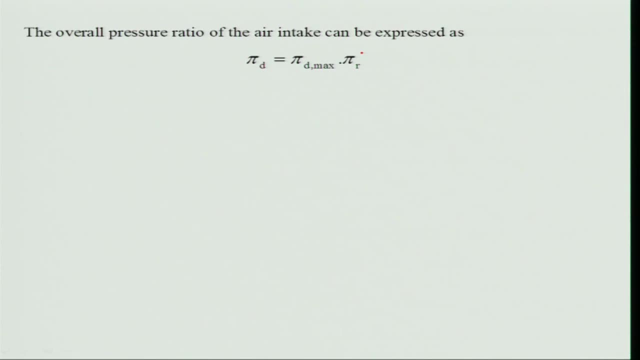 know, because particularly in supersonic flow, the ramming effect will be very, very high and this pi? r in the subsonic flow, or the low subsonic flow, will be almost equal to 1. we will see that. So the pi d maximum, certain portion of ram. 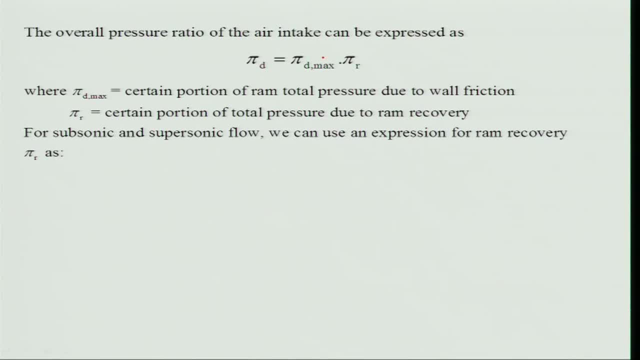 total pressure due to wall friction, because wall friction will be there. So therefore this value will be having certain thing which is due to wall friction, whereas pi? r certain portion of total pressure due to ram recovery. And now to get this pi? r is not that easy. 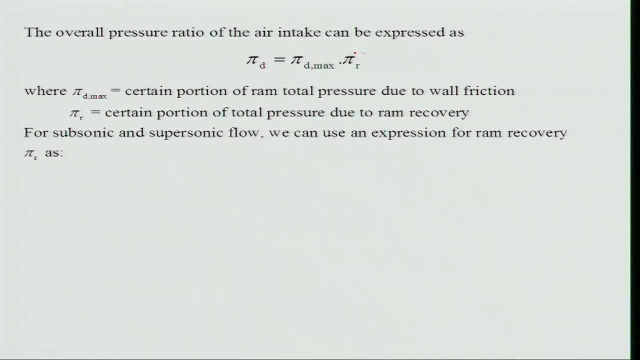 what we will be using, an empirical relationship which, of course, was being derived long time back in may, be in sixties. that till we are using pi r is equal to 1 and m net, you know, less than equal to 1, very, very low subsonic or the subsonic value. 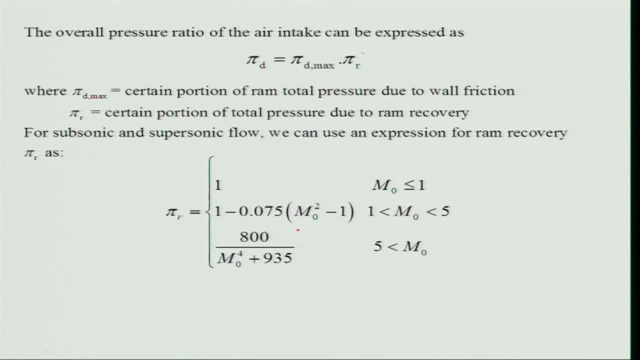 So this is what we will be using in the subsonic flow: right, it will go on. Whereas the m not 1 to 5, you will have to use this expression, and when the m not, you know, is beyond 5, you will have to use this expression. right, particularly supersonic, very, very high, rather hypersonic. 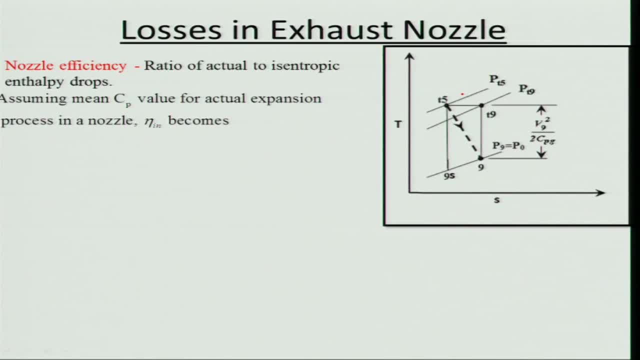 your turbine. If air intake will be there, then it will be t, t, 7, right? sorry, if the after burner is there, there will be 5 to 7. is the this thing: 7, 8, 9, right? So it is, we can say: 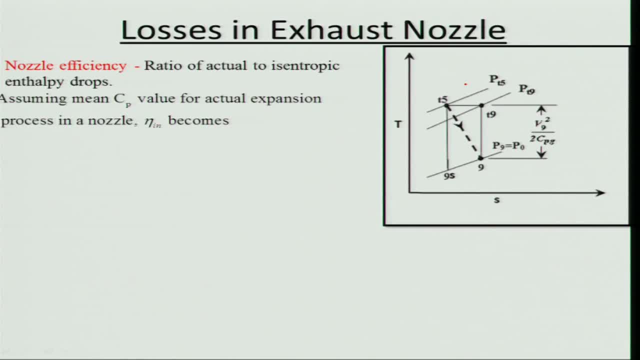 either it is t 7 or t 5 right, both are same. So if we look at dimensions after burning area t t 5, then actual expansion will be from t t 5 to t 9.. Whereas the isentropic expansion will be t? t 5 to t 9 s right. t 9. 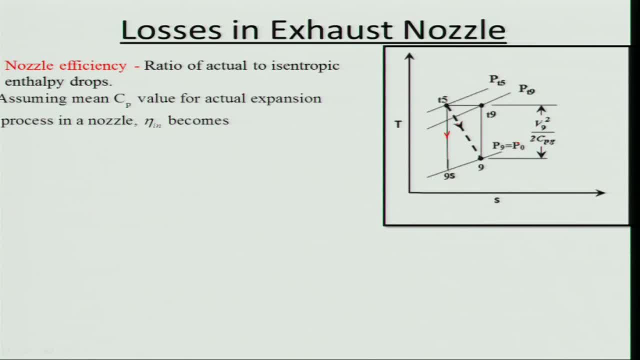 s, but the pressure remains same. t 9 is equal to t naught that we are considered. But when I will talk about the what you call turbojet engines, then will be talking about choking condition, whether it is choked or not, right? 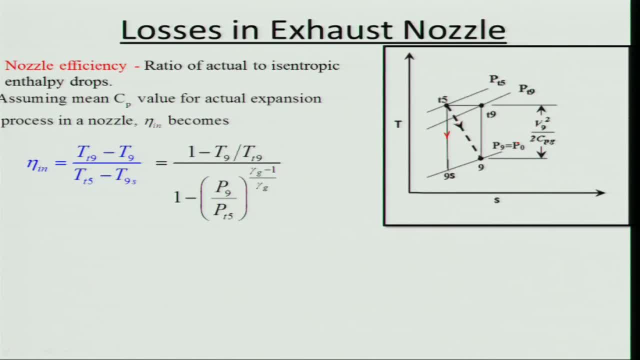 let us define this nozzle, efficiency, that is, and keep in mind that this is the same. this is t t 5 is equal to t t 9, because adiabatic. we are considering therefore t t 9 minus t 9, divided by t t 5 minus t t s, and if I divide this by the, you know, t t 9 and divide: 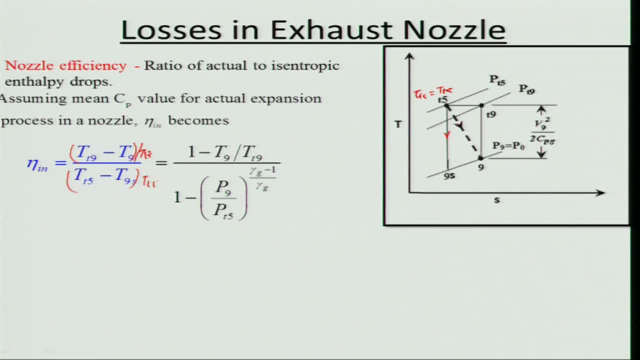 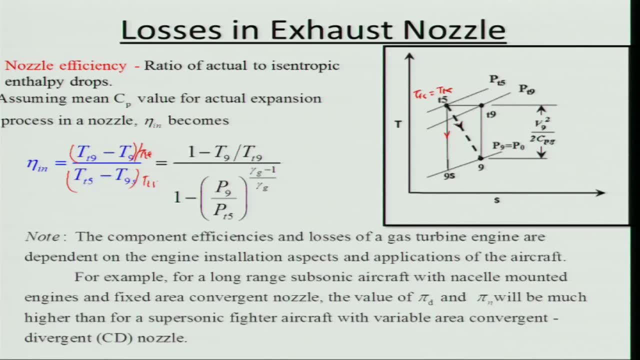 by the t t 5, which is basically same right. So you can get this thing and this is a ratio, you know, and we will be getting all those values, and we can express this: t t 9 s by t t 5 in terms of pressure ratio: p 9 by p t 5. power to the gamma g minus 1 divided by 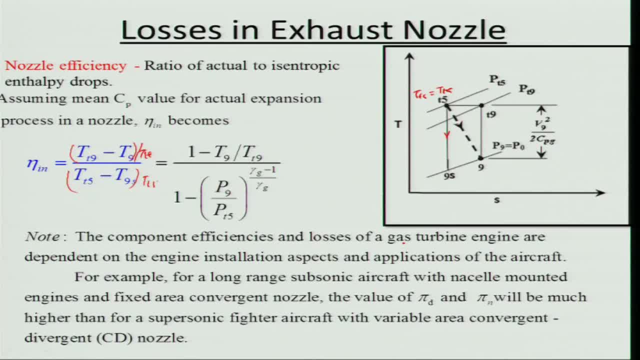 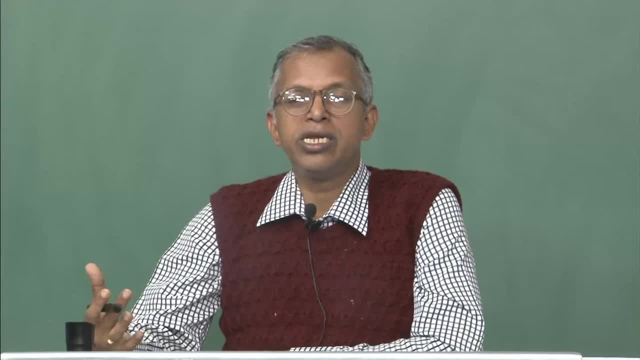 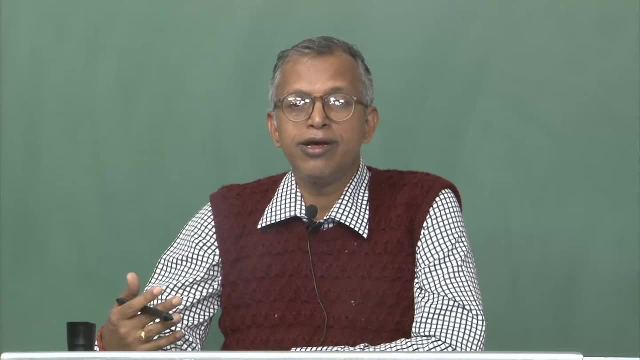 gamma g. The component efficiencies and losses of a gas turbine are dependent on the engine installation. So different aspects and applications of the aircraft, because the different installation of the engine will be having different efficiencies. right, For example, in fighter aircraft you install the engine in the adjacent to the fuselage is a part of fuselage, whereas in 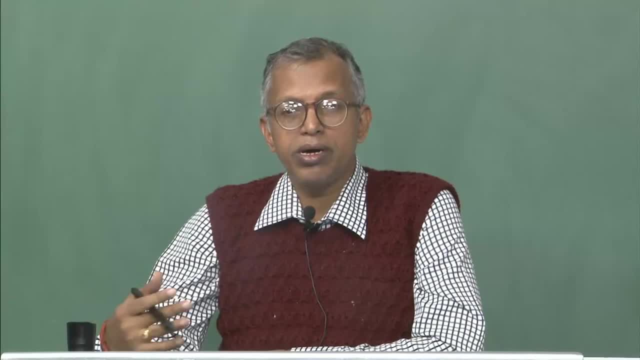 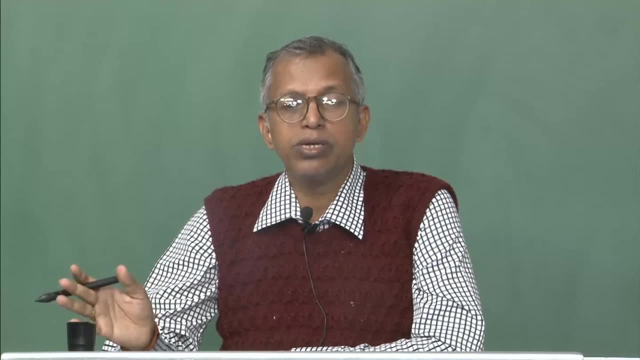 other places it is like a pod. it will be hanging from the, your wing, So naturally it will be. in some cases you may put on the on the back side of the fuselage, So therefore, what you call it will be having different efficiencies.